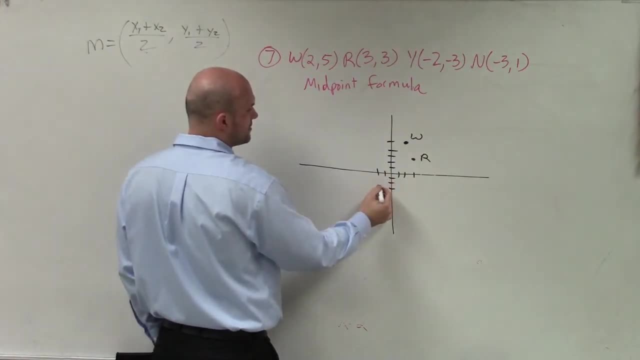 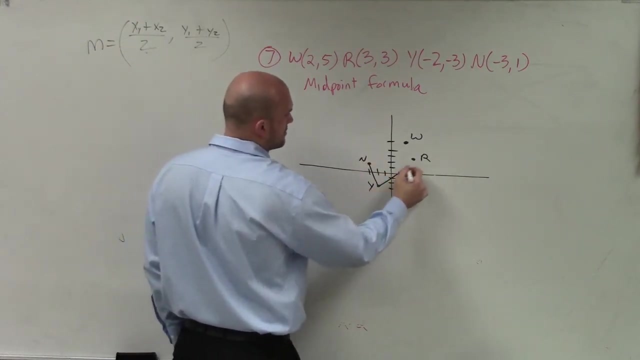 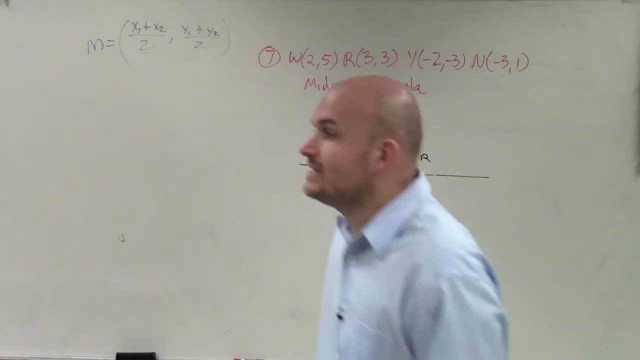 y is at negative 2, negative 3, 1, 2, 3.. And n is at negative 3, 1.. OK, so that's what our parallelogram looks like, And what we need to do is determine. 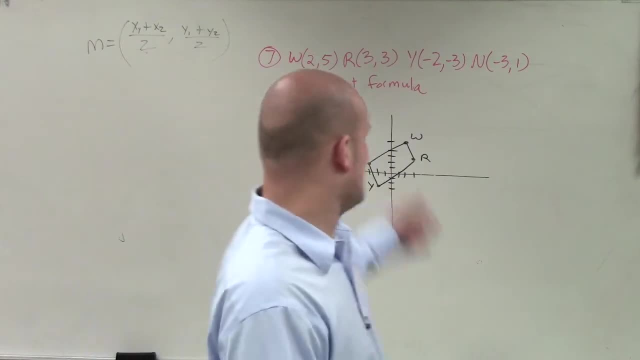 is that parallel Parallelogram? Well guys, just because, oh yeah, that looks like a parallelogram, so, yeah Or no, it doesn't look like a parallelogram, That's not going to be a good enough reason. 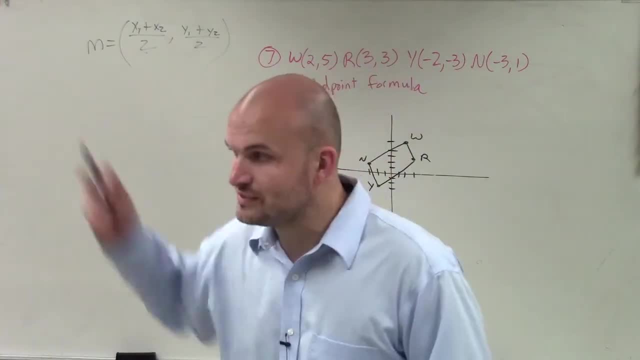 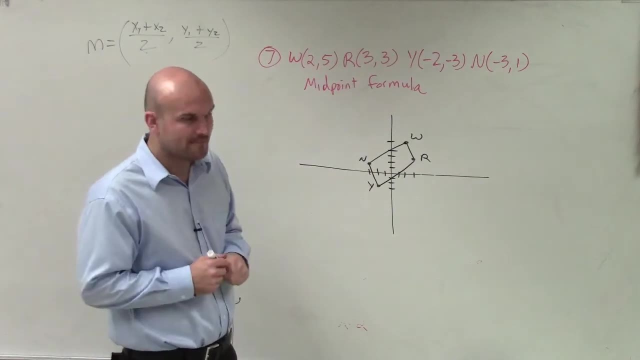 What we're going to have to use is use our properties of parallelograms, which we've talked about before, But they want us not only to use any property, but they want us to use a property stating the midpoint formula. So what we're going to want to do is remember, guys. 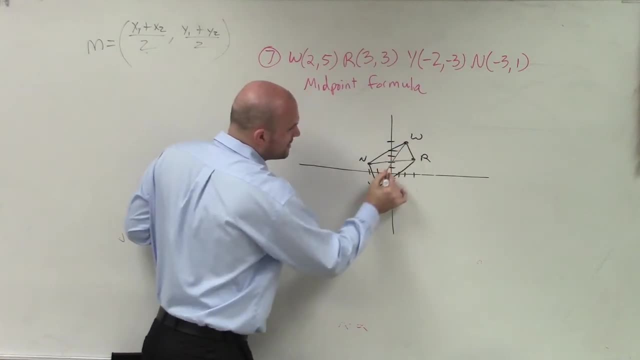 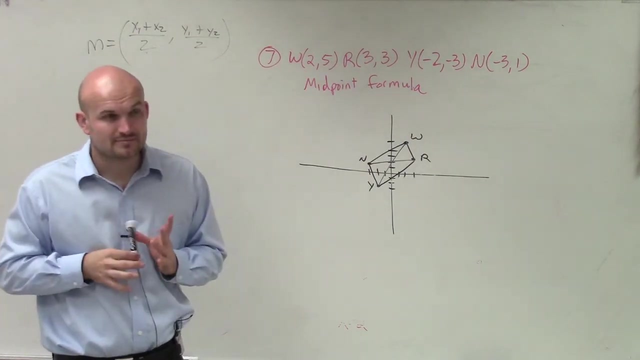 when we talked about parallelograms. what is one thing that we knew about the diagonals of a parallelogram? Dustin, do you remember one thing about the diagonals of parallelograms? They bisect each other. They bisect each other. 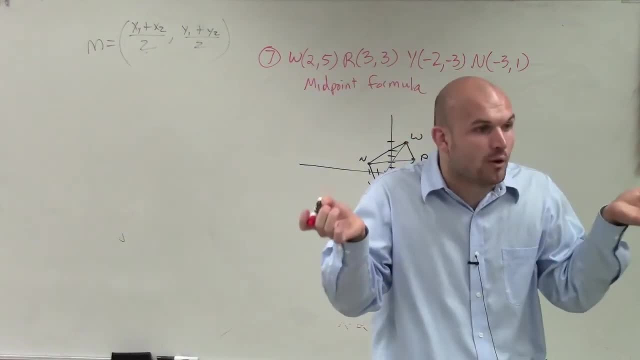 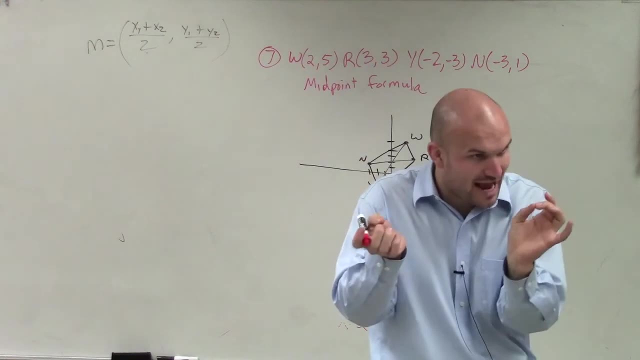 That means they cut them in half, right? If I said: find the midpoint of a line, where would that midpoint be? In the middle right? Would that midpoint cut them in half? Yeah, cut the angle in half. So could you say if I have a line that bisects it. 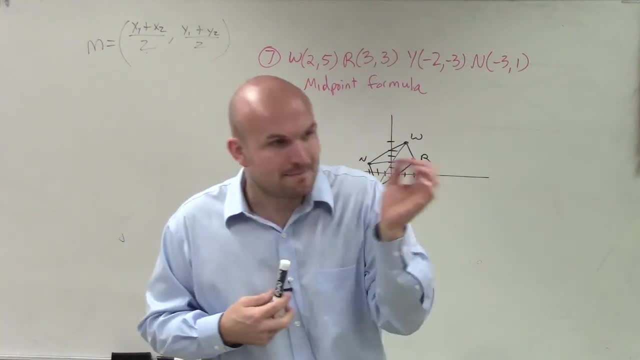 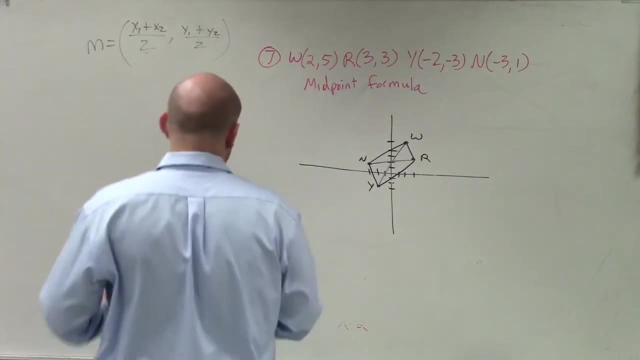 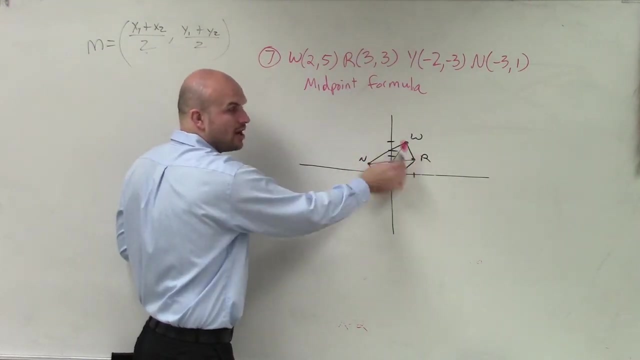 where that line bisects the other diagonal. would that be where the midpoint is? Yes, So I can prove that this is a parallelogram if the midpoints of my opposite angles are equal to each other. So what I want to do? I don't like that marker. 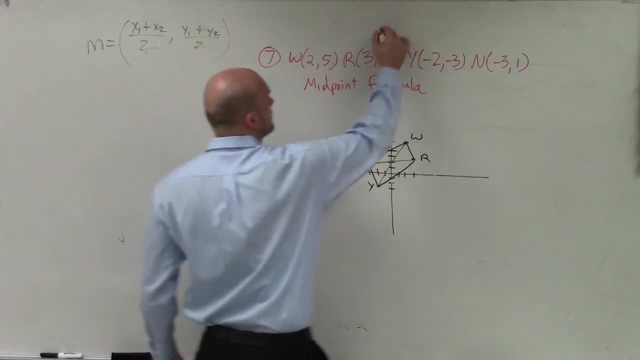 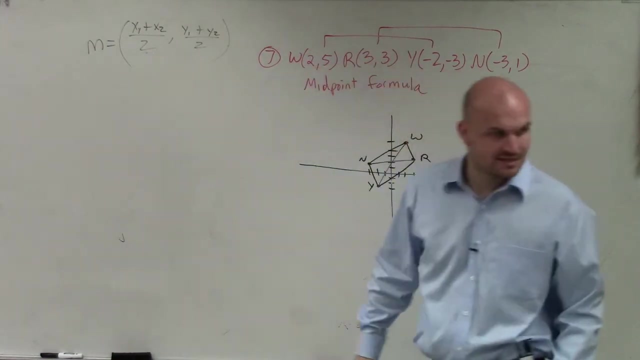 So what I'd like to do is: let's find the midpoint of nr and wy Now remember the midpoint formula which I gave you guys. even though you have to have this memorized, unfortunately for the end, I know you guys aren't going to use it. 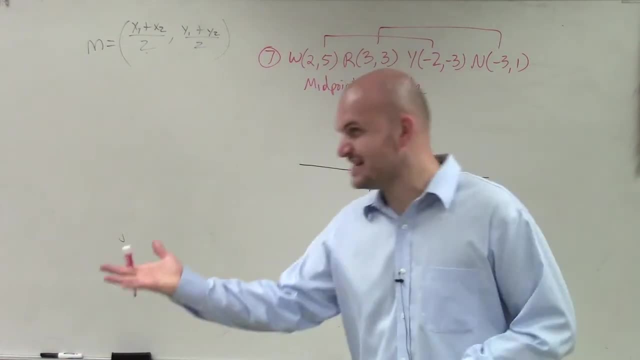 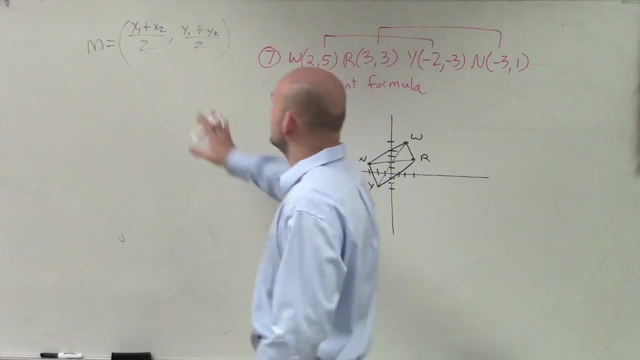 when you're texting your friends. It's not something you're going to send over to them. However, it is something that's kind of like your toolkit for this course. That's one thing we're going to be using over and over. So here's the midpoint formula. 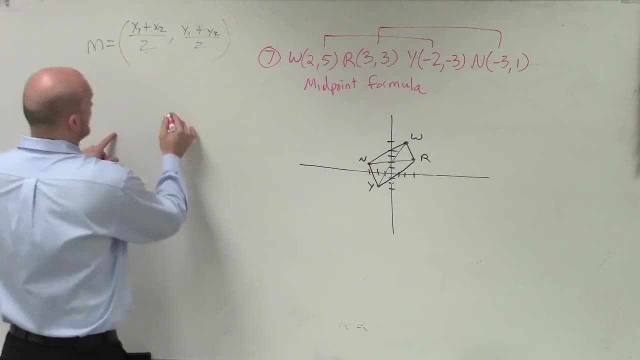 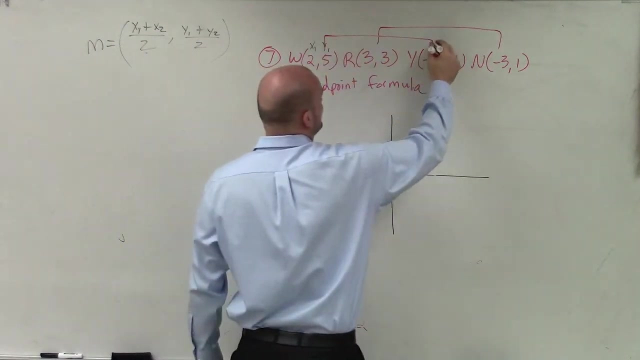 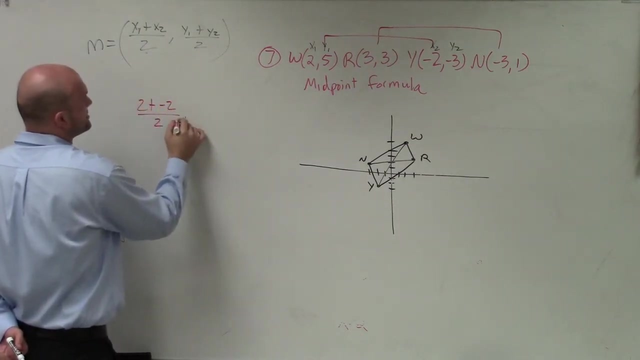 If I want to find the midpoint of w and y, I'm going to have x1. So I'll just label them. I'll label this as x1, y1. And I'll label this as x2, y2.. So I have 2 plus negative 2 divided by 2, comma 5 plus. 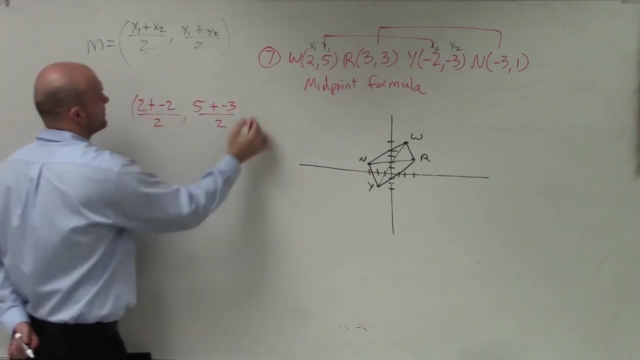 negative 3 divided by 2.. And this is for the midpoint of wy. So 2 plus negative 2 is 0.. 0 divided by 2 is 0, comma 5 plus negative 3 is 2.. 2 divided by 2 is 1.. 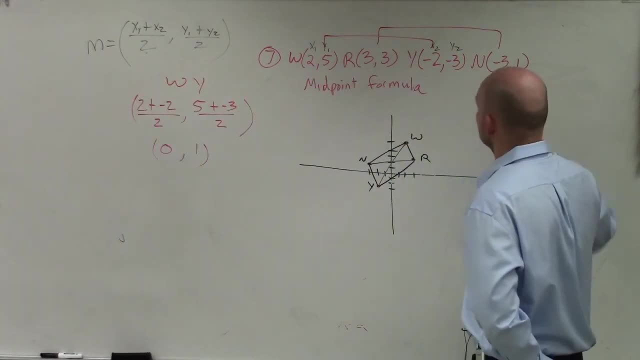 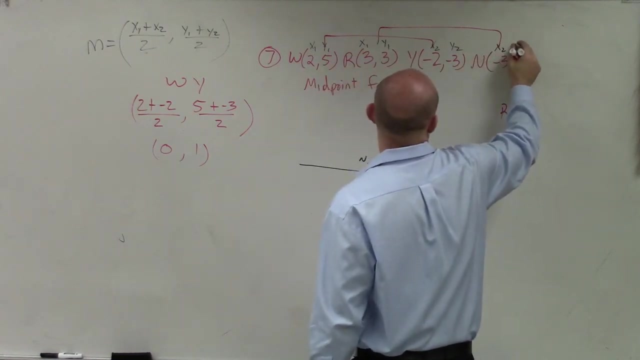 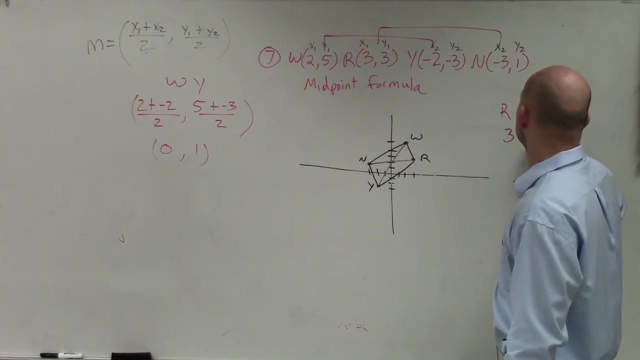 Now let's find the midpoint of rn. So I have- let's go ahead and label this now: x1, y1, x2, y2.. So here I'll have 3 plus negative, 3 divided by 2, and comma 3 plus 1 divided by 2.. 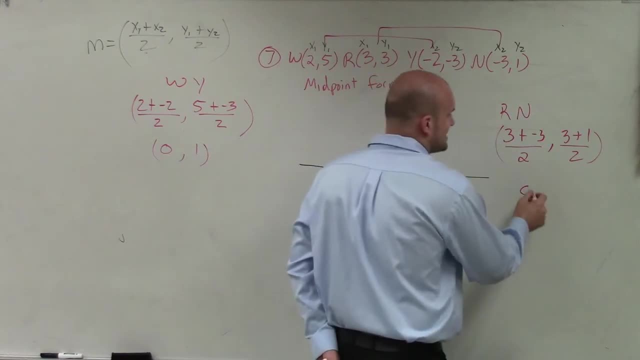 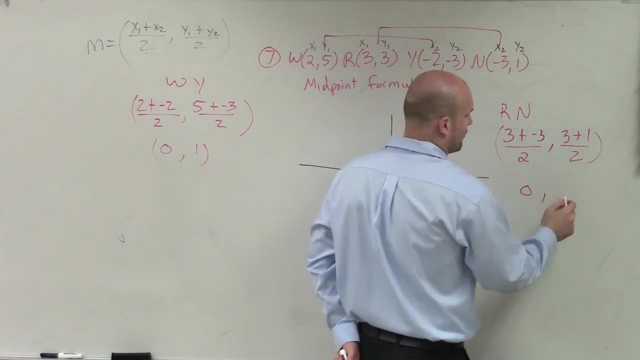 3 plus 3 is 0.. 0 divided by 2 is 0.. 3 plus 1 is 4.. 4 divided by 2 is 2.. Oh, that's 4.. 4 divided by 2 is 2.. 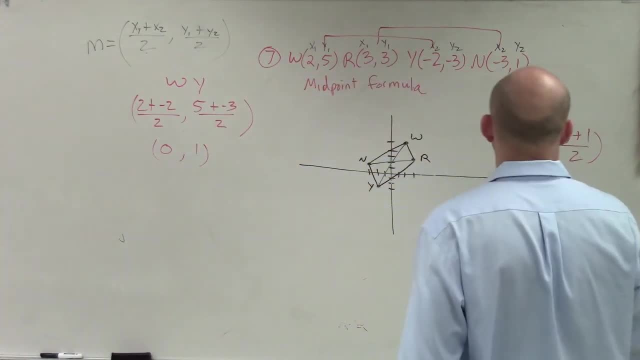 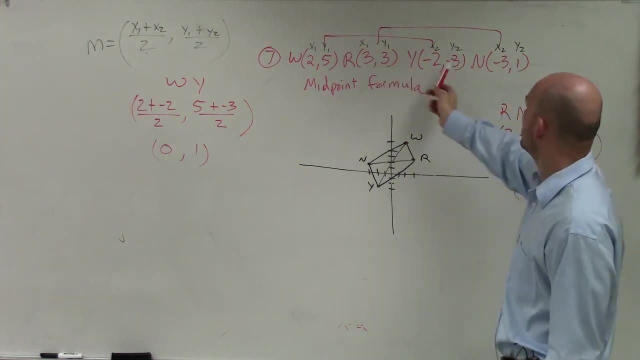 Did I do that right? No, I didn't. x wait a minute. that one and that one, right? Yeah, What? Oh? and 3 and 3, right, x1 plus x2.. y1 plus y2.. 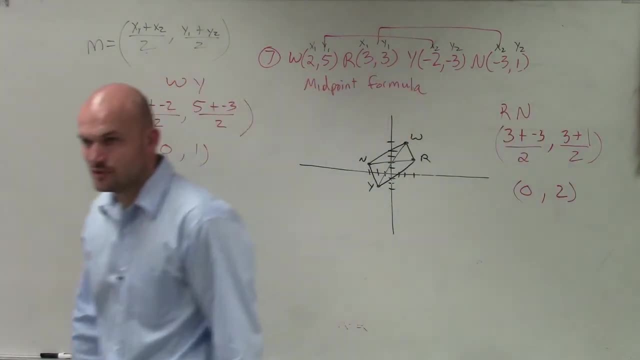 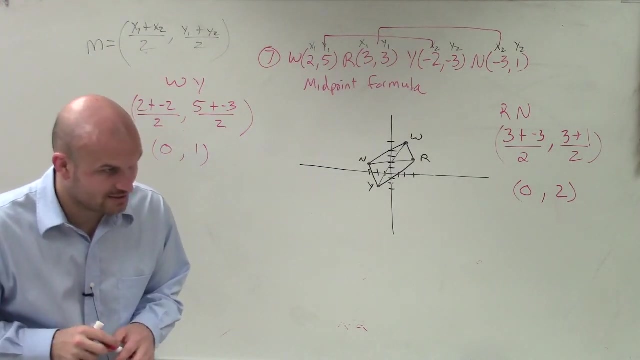 No, I was right. 3 and 1.. So do they have the exact same coordinates? No, So therefore their midpoints are not the same. Therefore, Taylor, this is not a parallelogram. OK, It's not a parallelogram. 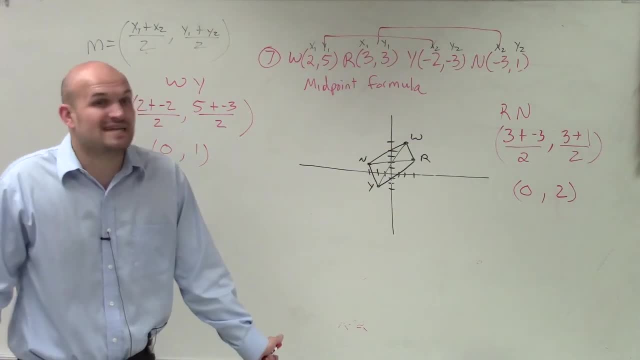 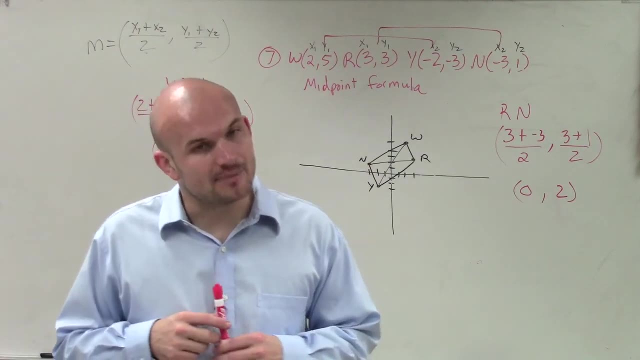 They do not share the same midpoint of their diagonals, Therefore their diagonals don't bisect each other And therefore they're not a parallelogram. Yes, No. So you can say: no, it's not a parallelogram. 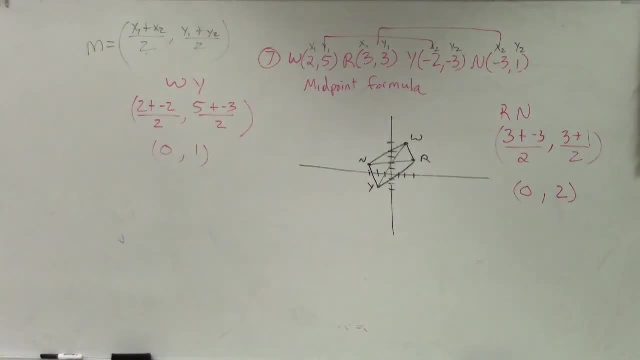 No, it's not a parallelogram. No, it's not a parallelogram.